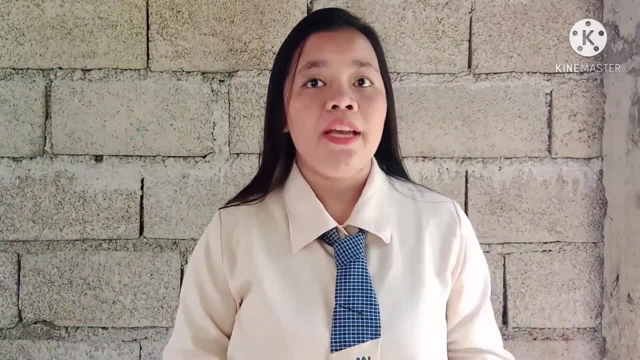 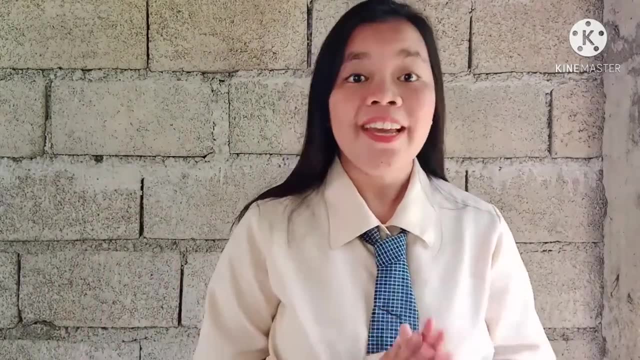 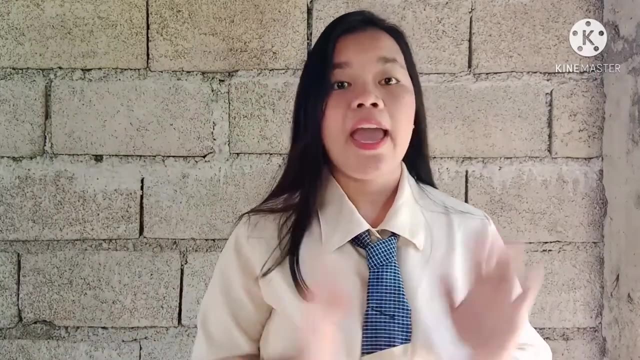 information is intended, can read and process it. The prefix crypt means hidden or bold, and the suffix graphy is that for writing. But wait, there's more. In addition to cryptography, number theory has been applied to other areas such as error-correcting codes, numerical integration, computer arithmetic, random and 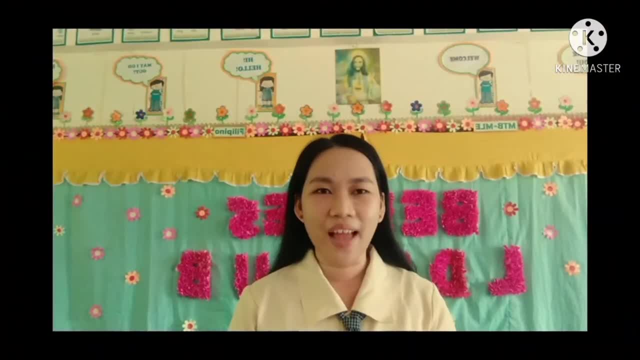 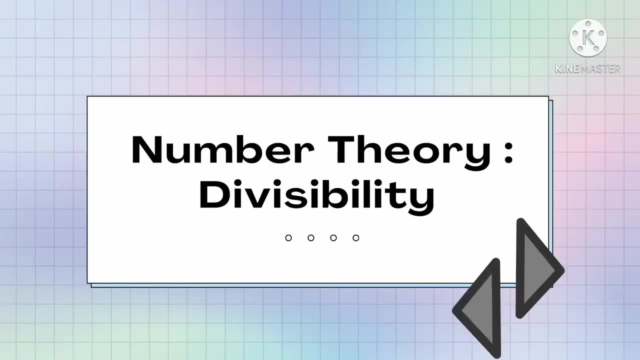 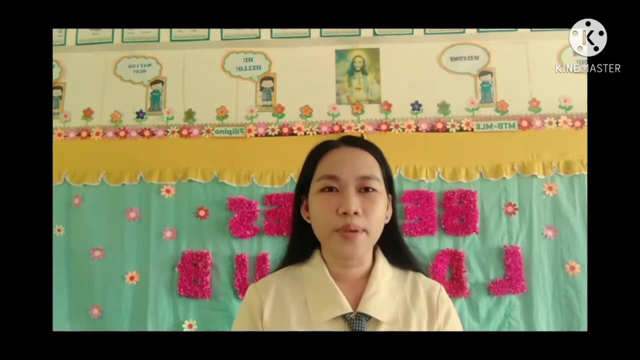 quasi-random number generation. Number theory is the best useful in our lives. Now let's continue discussing one of its concepts: the divisibility. Here's the definition of divisibility: A and B are integers and there is some integer c, such that a is equal to b times b, where a and b can be any. 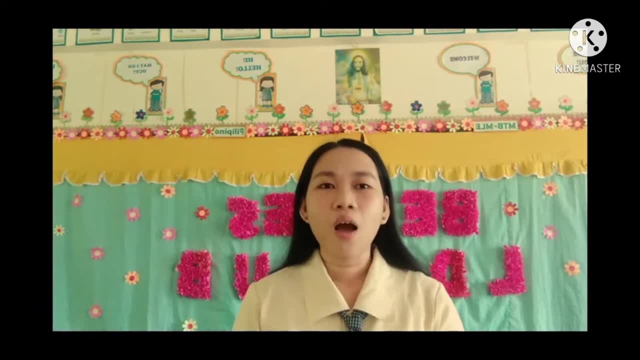 integer, but c has to be a factoid integer. Then we say that b divides a or b is a factor or divider of a. Then we write b divides a. But what do we mean by that? It simply means that the disability rules are tools. 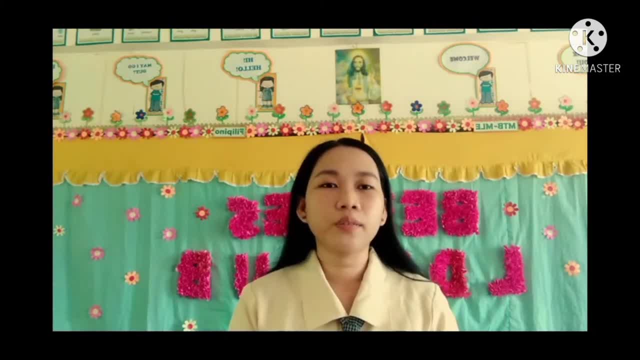 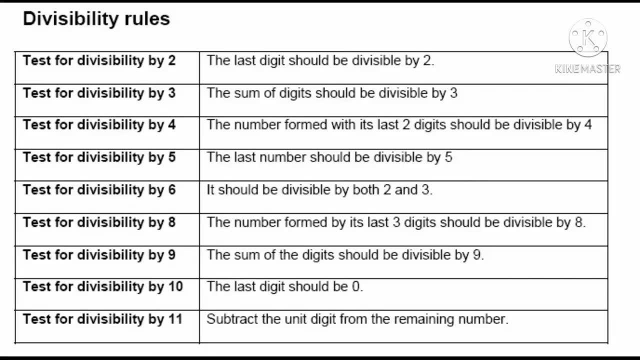 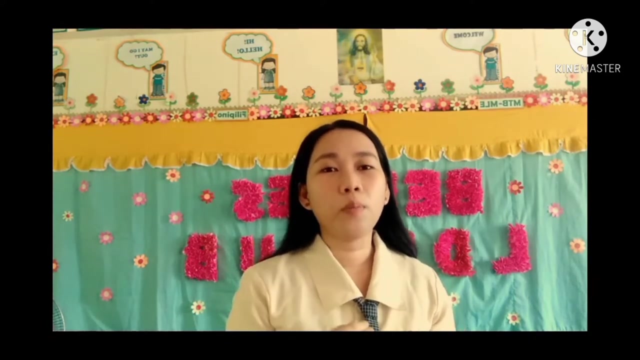 that helps you know quickly if a number is divisible by a certain integer. The following are few sample rules. Did you know that divisibility rules are useful in our life How? Let me give you a very common example. Divisibility rules can be used in everyday life. 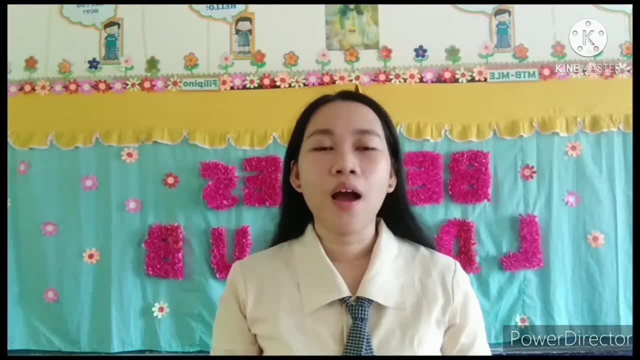 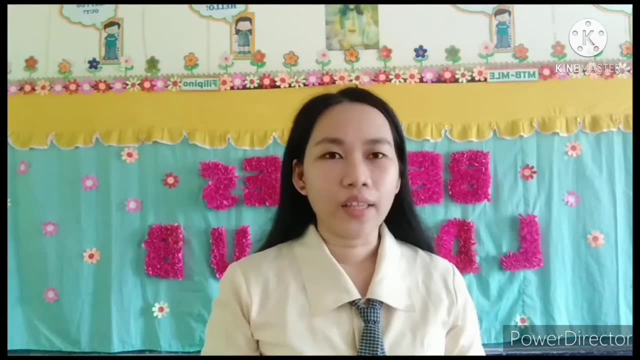 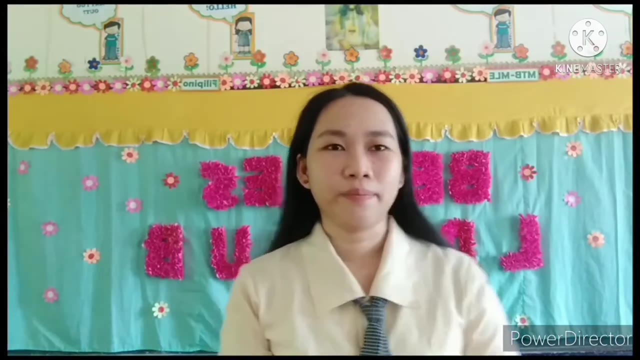 For example, if you're at a grocery store and need to find which deal is better using divisibility rules, Let's say, 2 cans of beans cost $6, while in another store 4 cans of beans cost $8.. Which deal is better? 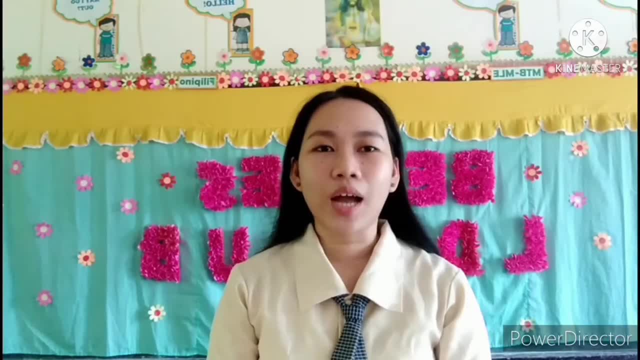 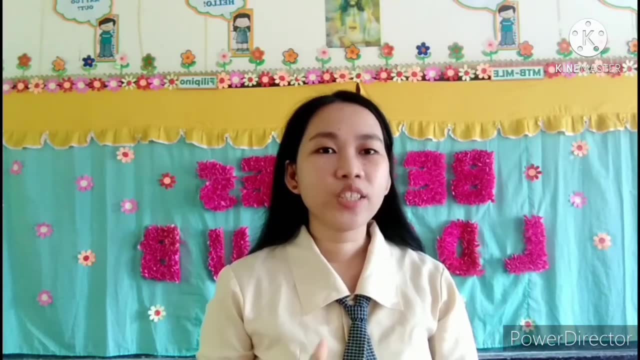 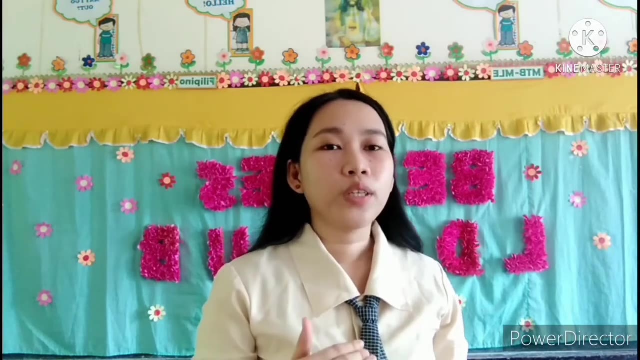 We know that 6 is divisible by 2, so each can cost $3.. We also know that 8 is divisible by 4, so meaning each can cost $2.. Now we know that the store with 4 cans, which cost $8, is the best deal. 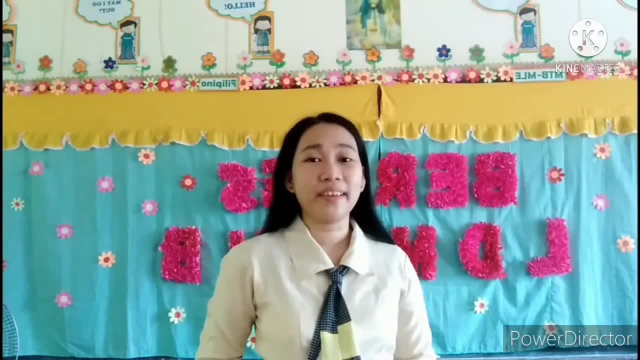 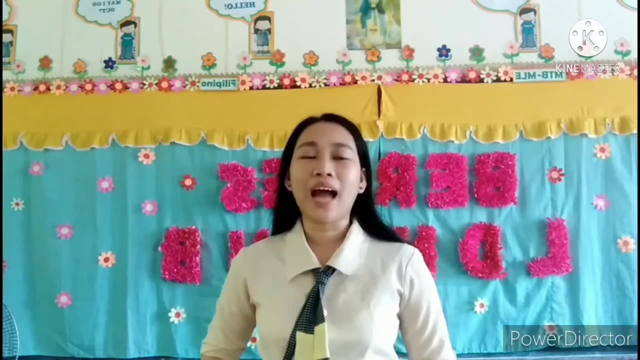 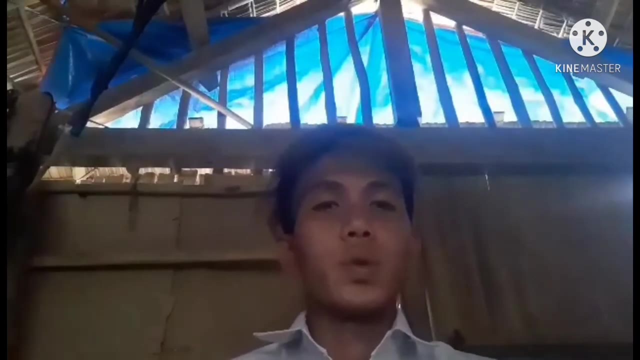 Can you now see how important divisibility is? There's a lot more uses of divisibility and we are actually using its concepts without us noticing it. We are done with the first concept, So let us proceed to the second one, which is congruence. 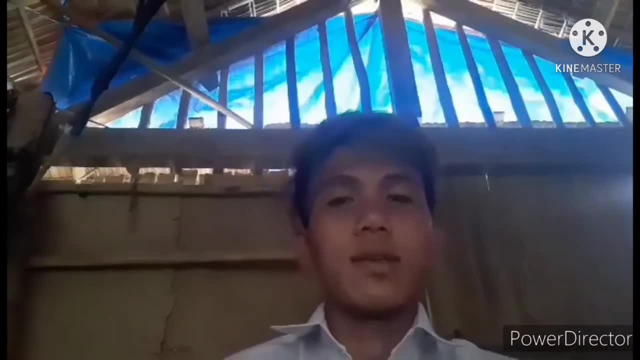 Proceed to the second one, which is congruence. Congruence is an important part and useful tool for the study of divisibility. As we shall see, they are also critical in the art of cryptography. Here is the definition of congruence. 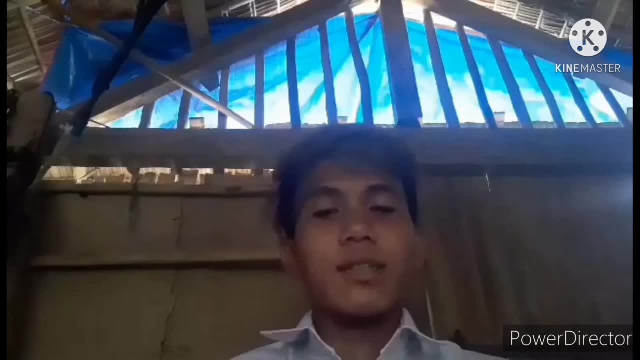 If a and b are integers and n is less than 0, we write: a is congruent to b modulo n, To mean n is divided by the difference of b and a. We read this as: a is congruent to b modulo n. 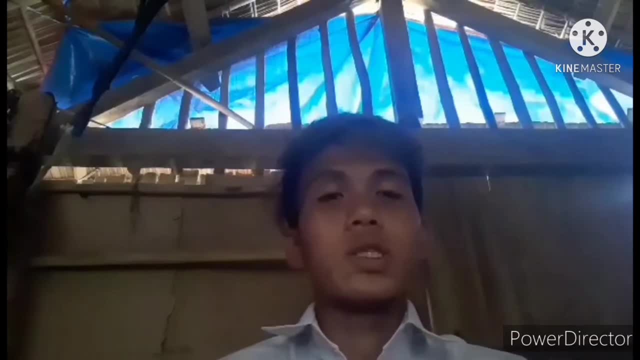 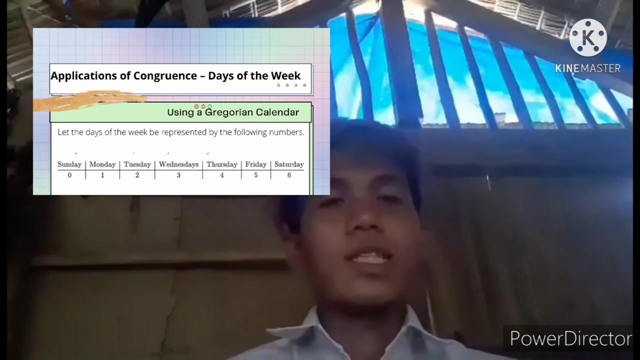 For example, 29 is congruent to 8 modulo 7 and 60 is congruent to 0 modulo 15.. We can apply the congruence in the days of a week using the Gregorian calendar. Let the days of the week be represented by the following numbers: 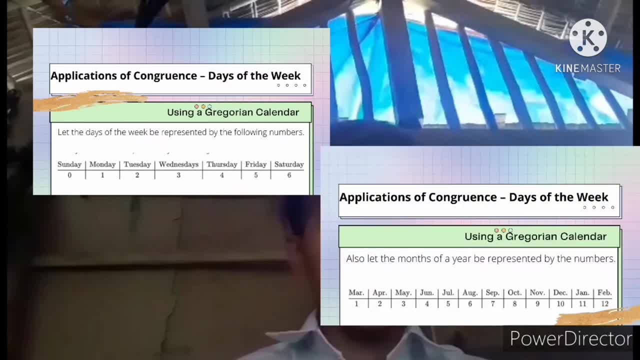 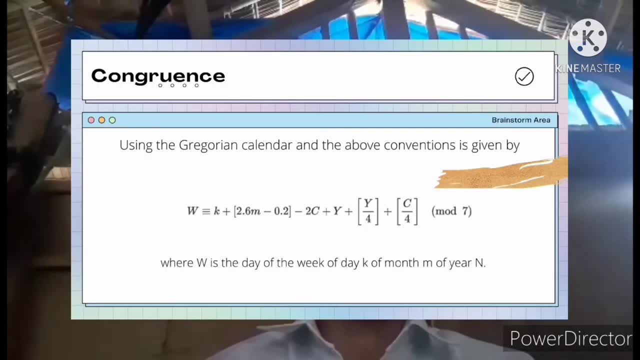 Also, let the months of a year be represented by the numbers. We can express each data using the following variables: Using the Gregorian calendar and the above, conventions are given Where w is the day of the week. w is the day of the week. 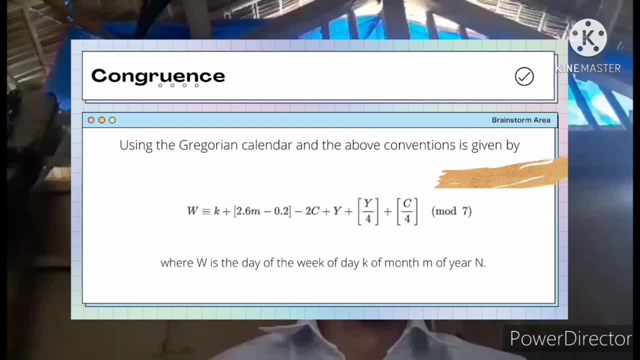 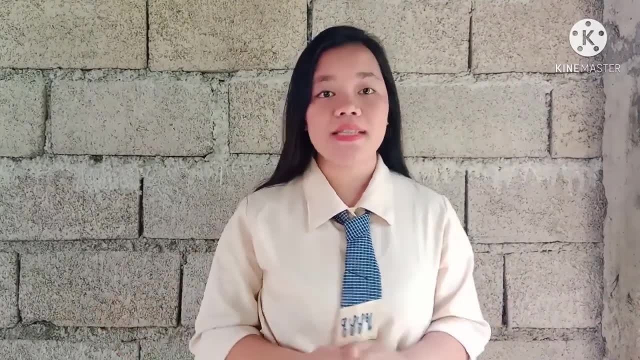 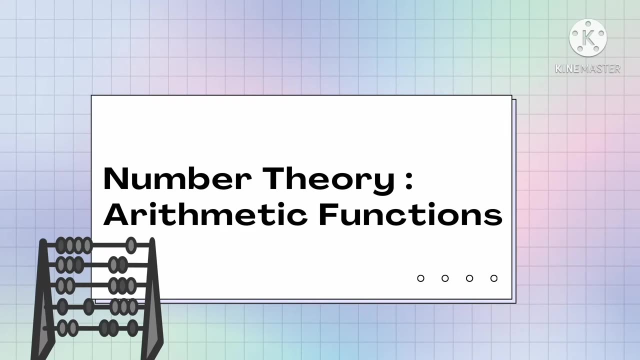 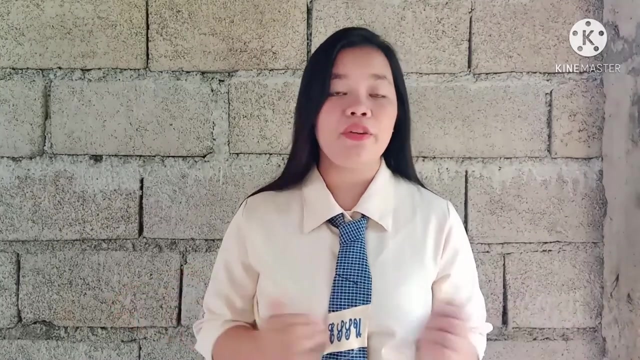 w is the day of the day, w is the day of the month. w is the day of the end of the year. We are now down to the last concept, which is the arithmetic function. An arithmetic function is a function defined in the passive integers, which takes values in round or complex numbers. 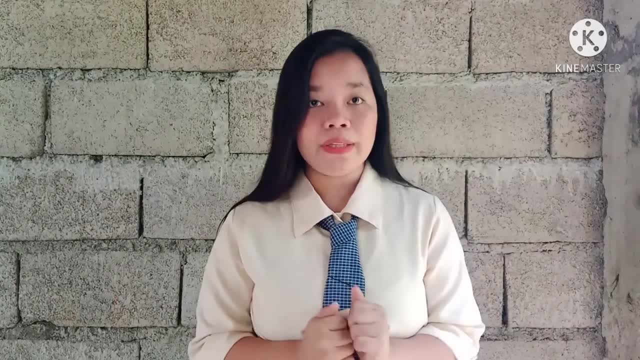 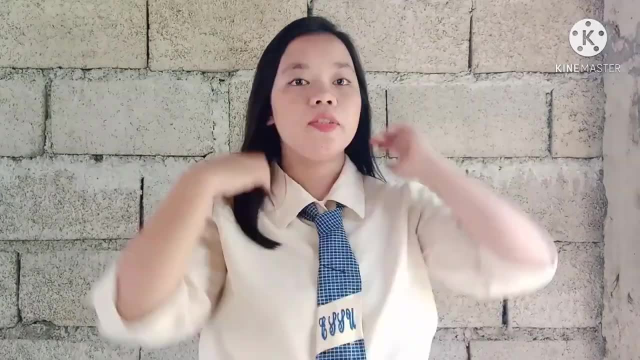 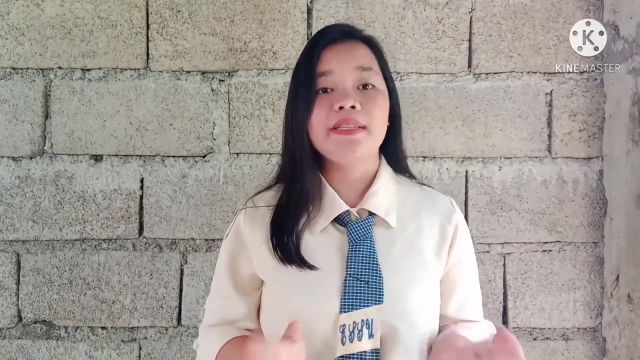 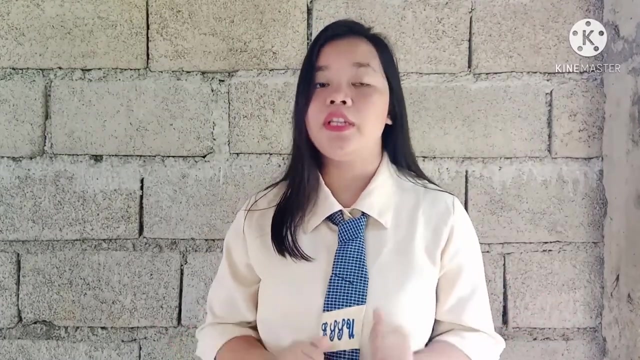 Many functions which are important in number theory are arithmetic functions. The Euler 5 function is an arithmetic function. Functions are everywhere where technology is literally, But since the world is not crazy about machine learning, let me mention this one. Machine learning is all about learning a function.